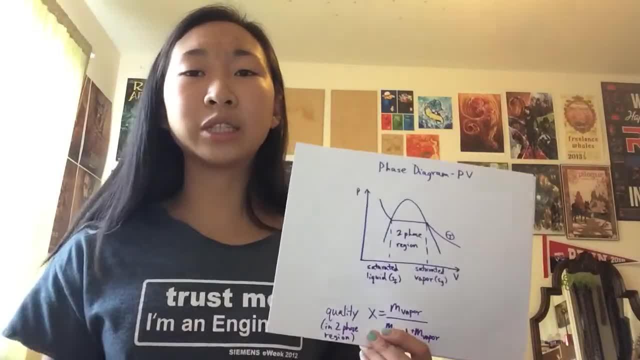 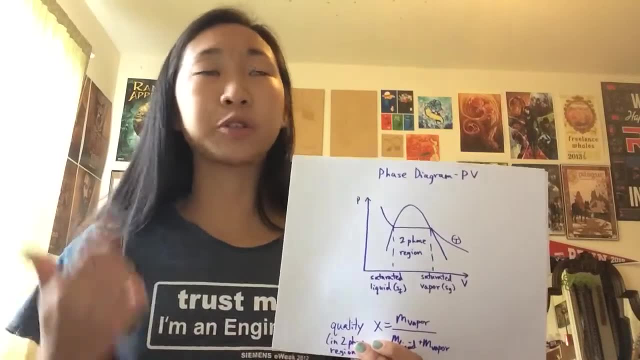 First of all, this vapor dome is the 2D representation, the 2D projection onto the PV diagram of this 3D PVT surface pressure volume temperature, a phase diagram that will show you the phase at any point on that graph. 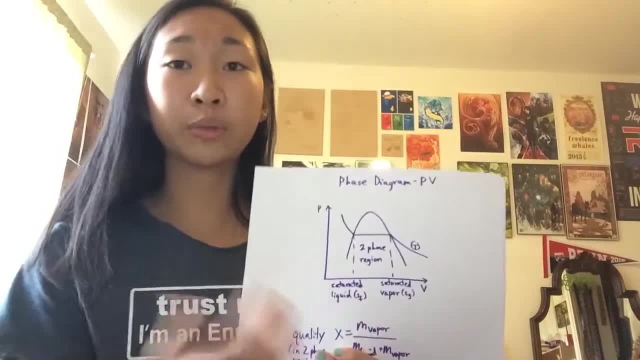 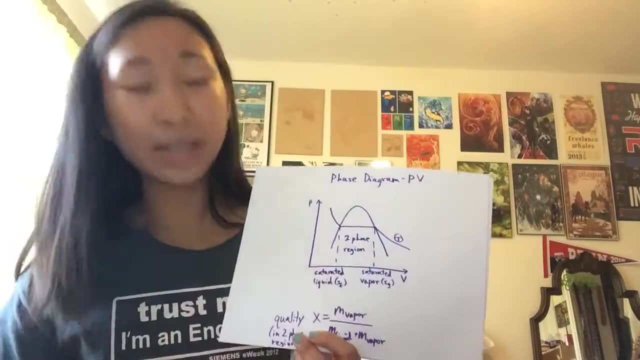 For example on this one, if you see where the isotherm intersects it, if you're at this point on the isotherm, along this left half of the vapor dome, anywhere on that point, you're a saturated liquid which can be denoted as SF. 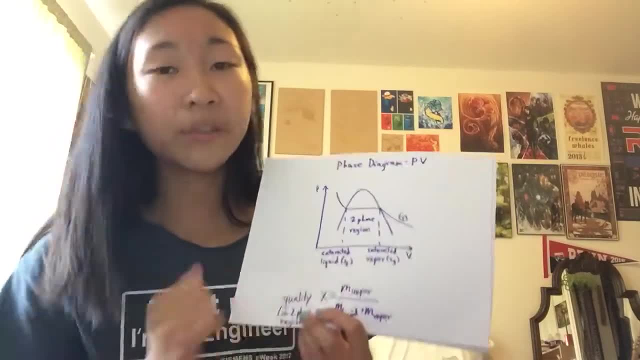 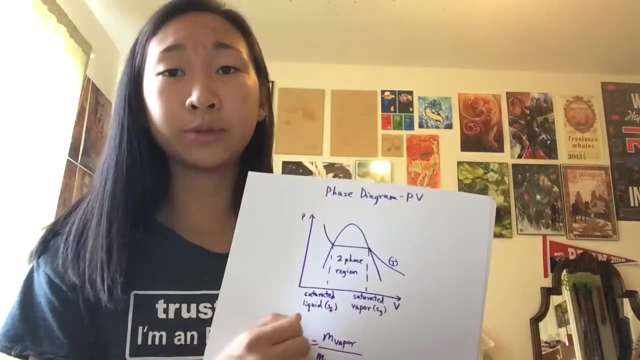 And once you get to the right you're a saturated vapor or SG. This isotherm at any point along this line, curved here horizontal across the two-phase region and then curved again down. there is at one temperature. 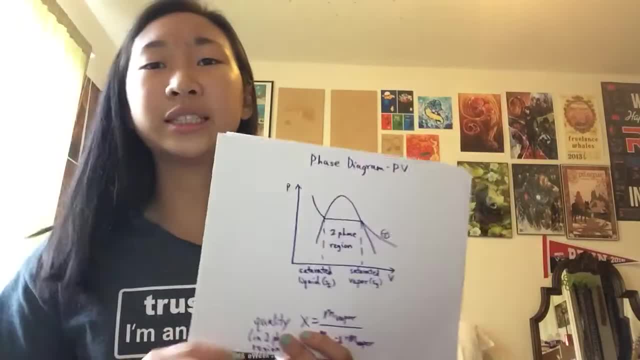 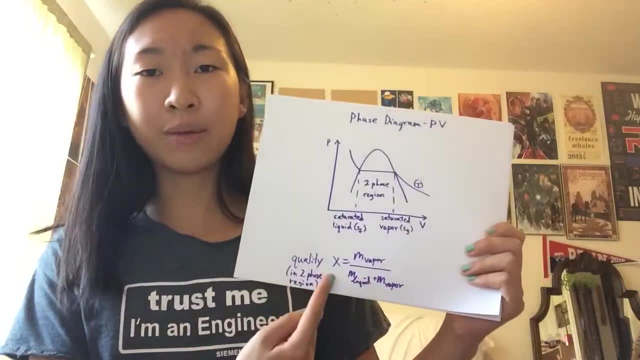 Once you get to the middle two-phase region, it's exactly that: two phases. So you have a mixture of gas and vapor. That's described with X, the quality at that point. So the quality is basically the ratio of vapor to the total mass. 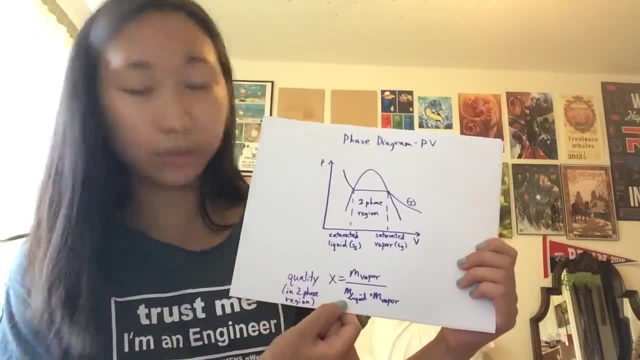 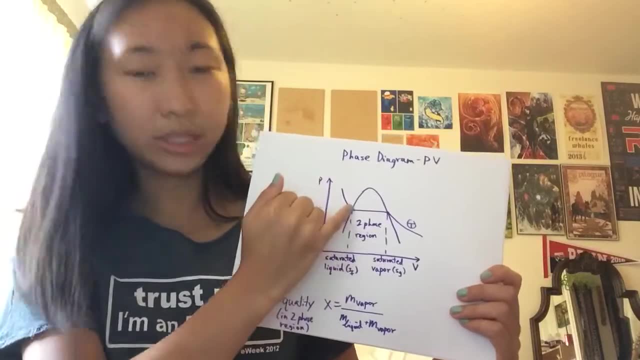 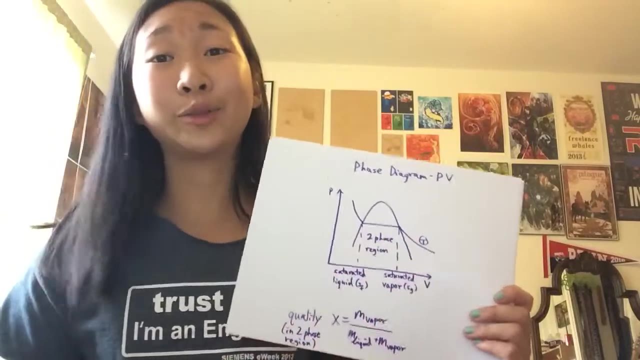 So you're going to have mass of vapor over mass of liquid plus mass of vapor On this isotherm. you'll start here, get to the saturated liquid at this point, increase in quality across the two-phase region and then, over here, you'll be saturated vapor and then vapor continuing onwards. 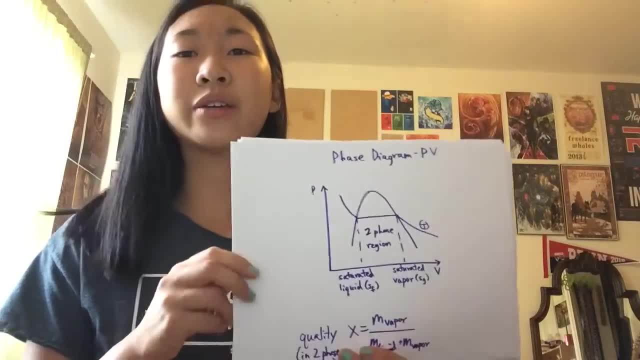 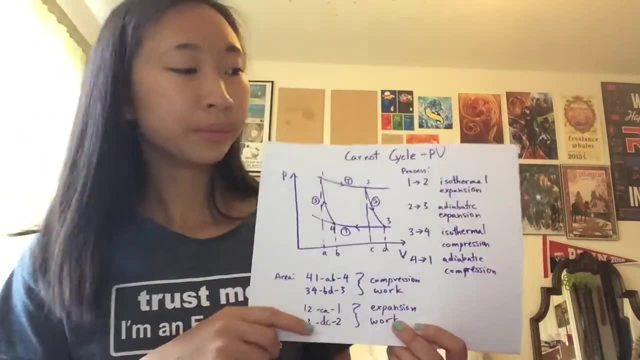 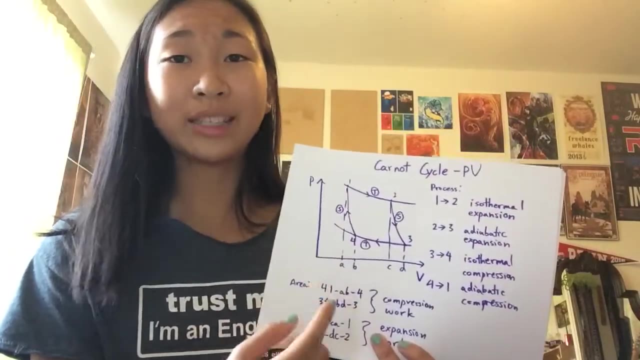 So those are the basics, Thank you. So these are the points on a PV graph that you will see. The most common system would be the Carnot cycle. Seeing this on a PV diagram, you're going to see some curved lines, but now you'll know these two curves are isothermal lines. 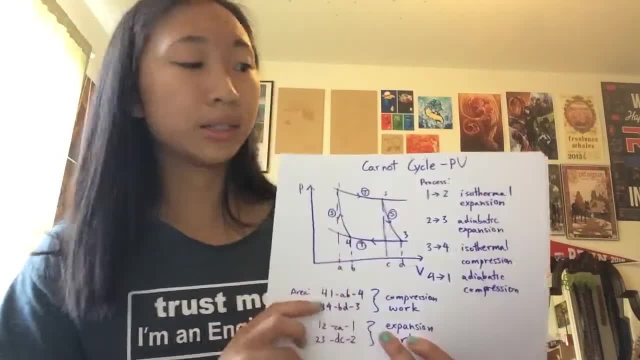 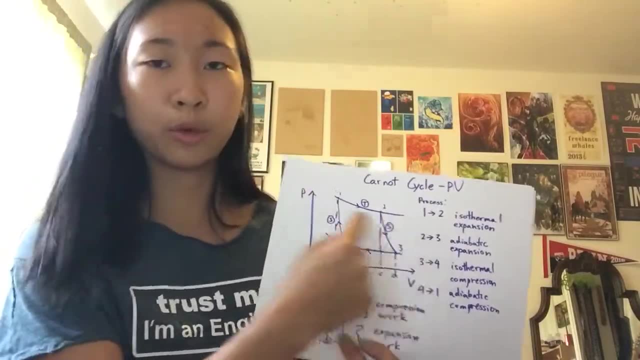 and the steeper inverse relationship would be the isentropic lines From one to two. it's an isothermal expansion. You can tell that because you're on an isothermal line here and increasing in volume. So going right on the diagram, 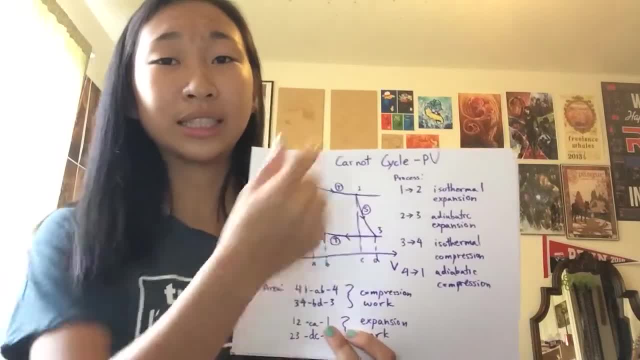 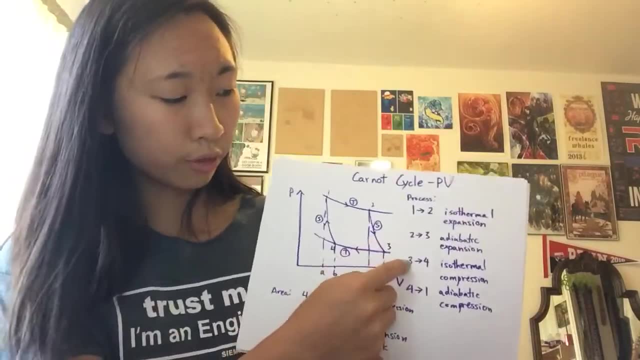 The second process would be an isentropic process, that's a steeper curved line that's also increasing in volume. Therefore, adiabatic expansion Three to four going backwards on the graph means you're compressing and being on a constant temperature line means it's isothermal. 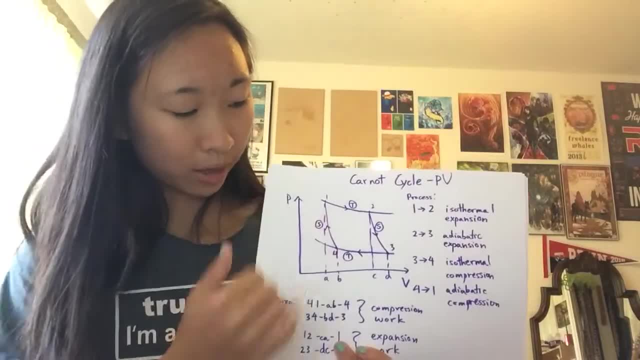 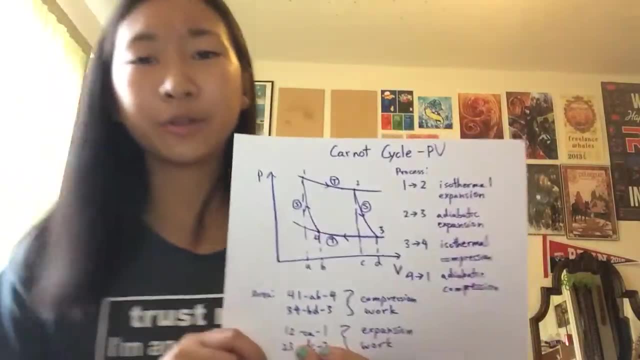 So you have an isothermal compression Going back up, you're going to have the steeper adiabatic isentropic line and a compression because you're still going left. on the PV diagram In total, you can see how these lines drawn represent this system. 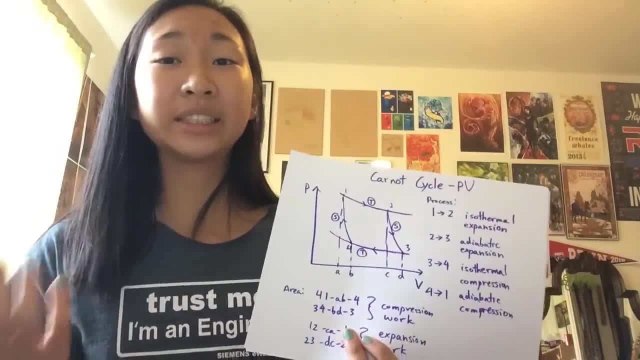 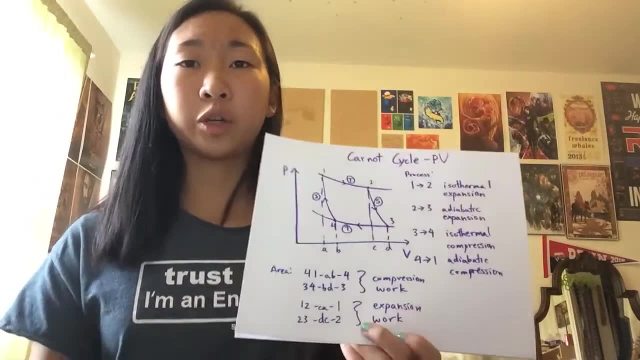 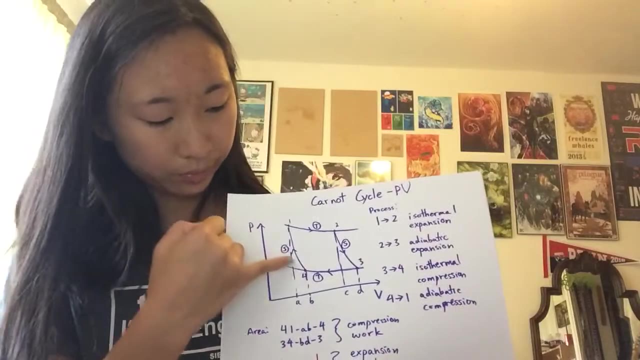 and the cycle being an idealized thermodynamic cycle, being easily drawn on a PV diagram. You can see and reference other Khan Academy videos, such as what are PV diagrams, to see a mathematical explanation of why the area under these processes, for example, 1, 4, B, A, 1, this little section. 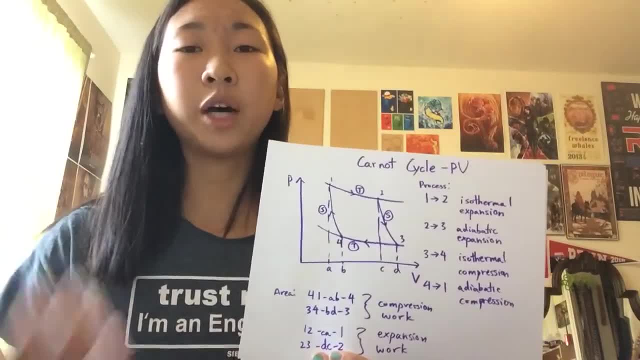 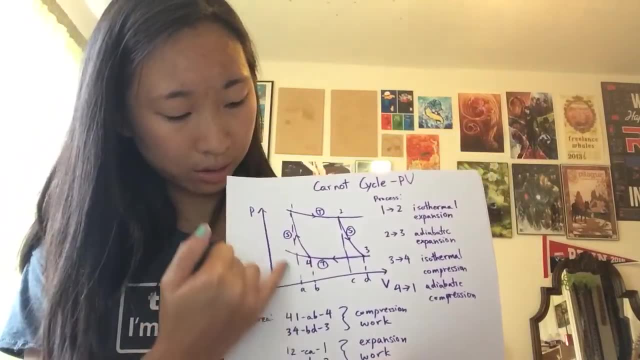 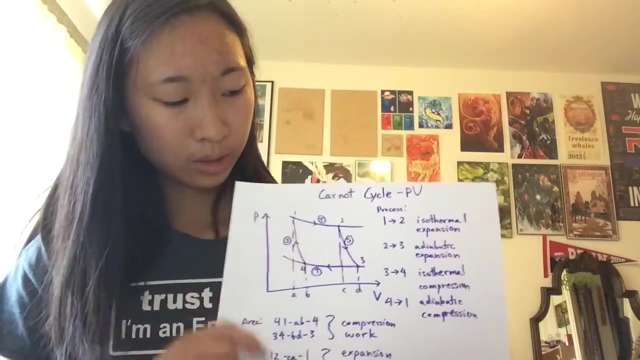 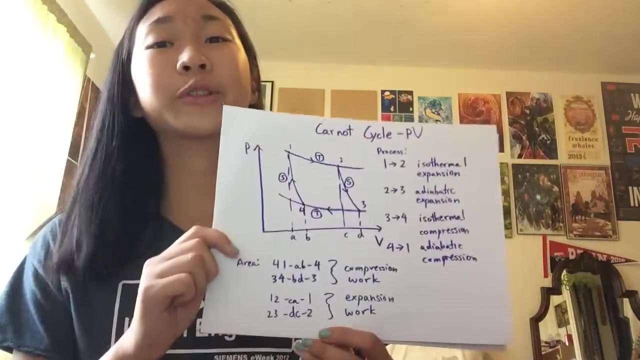 you can see why the volume under the curve represents work, In this case the part I just showed there because it's negative work would be compressive work. So in this cycle, these two compressive processes produce compressive work and the expansion processes create expansion work. 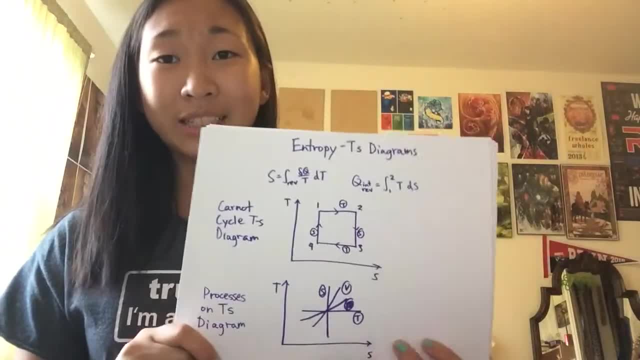 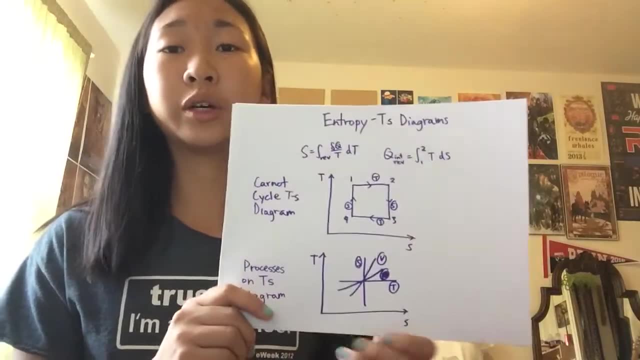 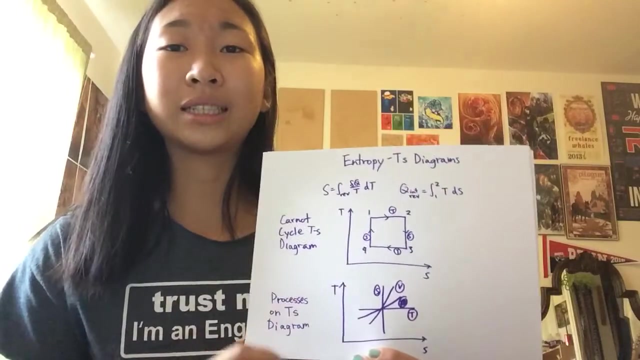 Cool On to the TS diagram. Entropy is usually a concept shown later in a thermodynamics course, but still a very important one. At that point you start drawing TS diagrams, or temperature versus entropy. You can see how it simplifies certain processes. 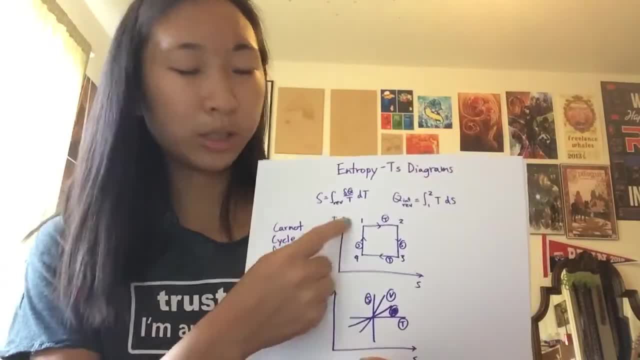 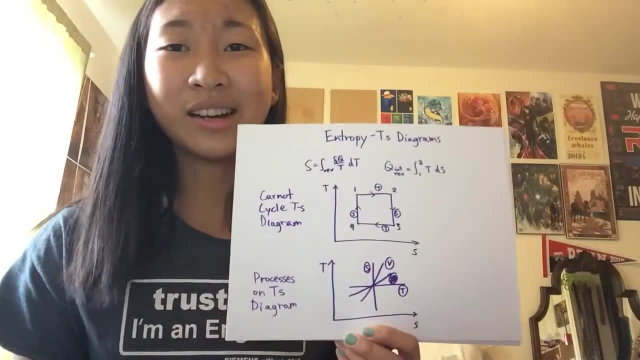 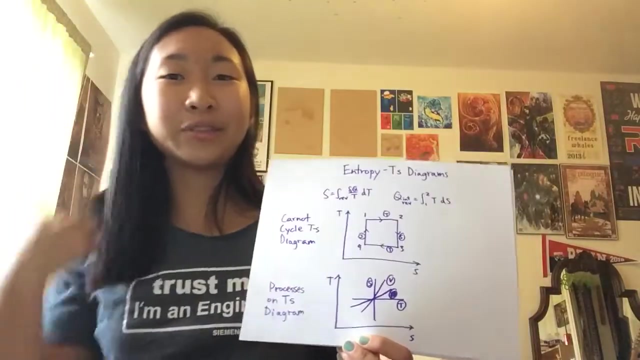 that are focused on entropy and studying that, such as the Carnot cycle, with a square or a rectangle which still shows two isothermal lines and then two isentropic lines. On a TS diagram, you're going to have the S, the constant S- isentropic line, as a vertical line. 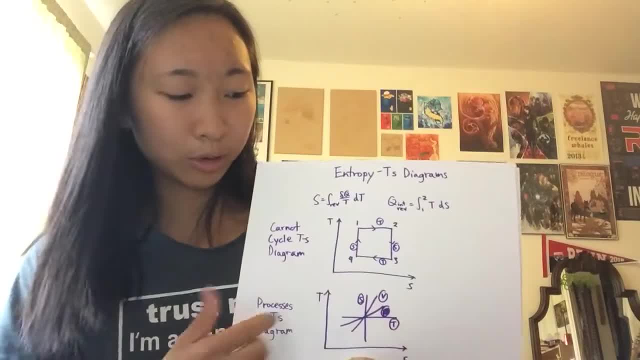 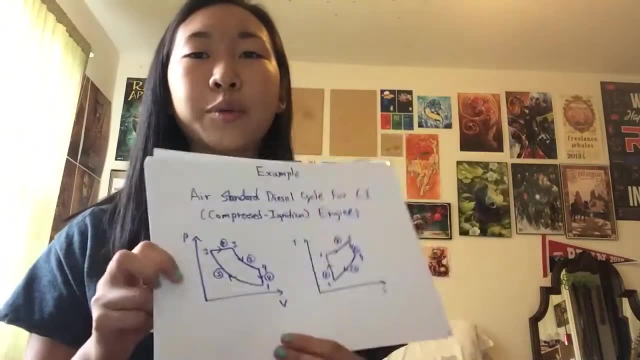 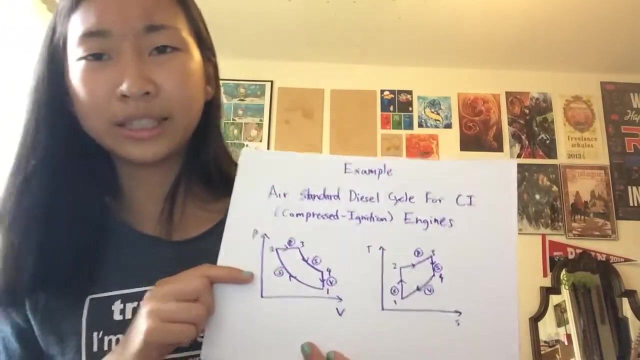 the isothermal or constant temperature lines as a horizontal line, and then the constant volume line being slightly steeper than constant pressure. Those common processes are shown in another example, which is the air-standard diesel cycle for CI compressed ignition engines. Basically, right now, you just need to pay attention. 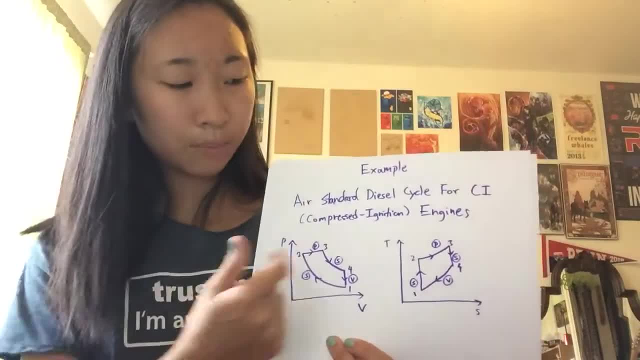 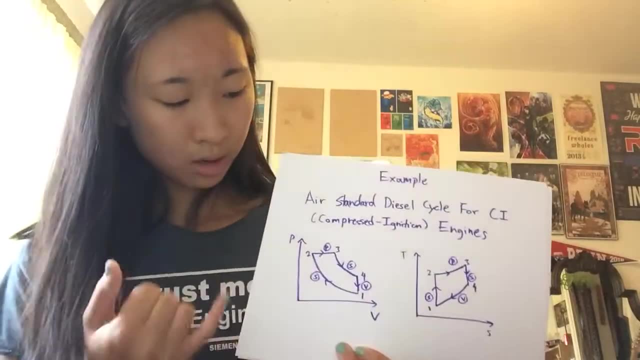 to the fact that it's air. so, since it's in the gas phase, both of these are shown on the right side of the vapor dome and does not need to be included. It's assumed you're on the right. On that side you can see the isentropic lines. 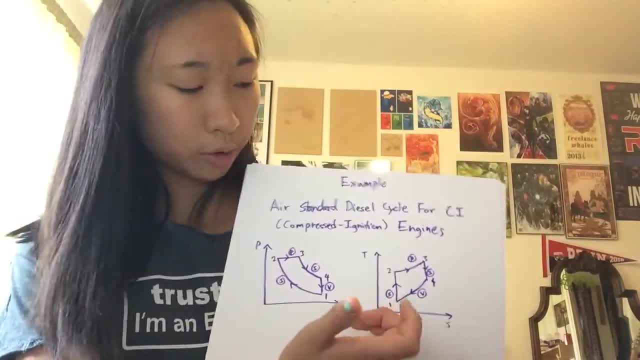 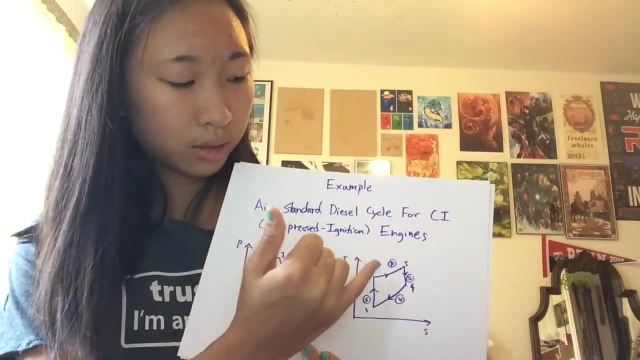 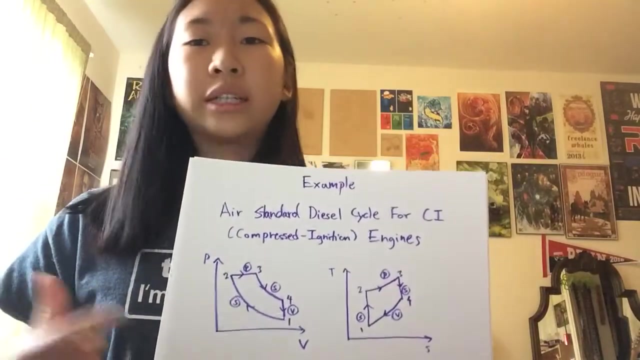 the constant pressure and the constant volume and how that translates over to a TS diagram which also shows the constant entropy lines, but also that the constant volume line is steeper than the constant pressure line. You can figure out work and a lot of different variables. 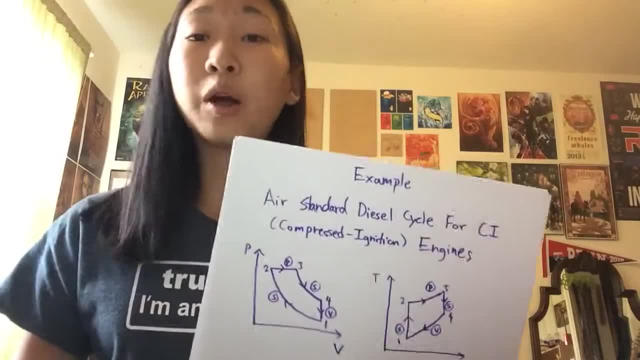 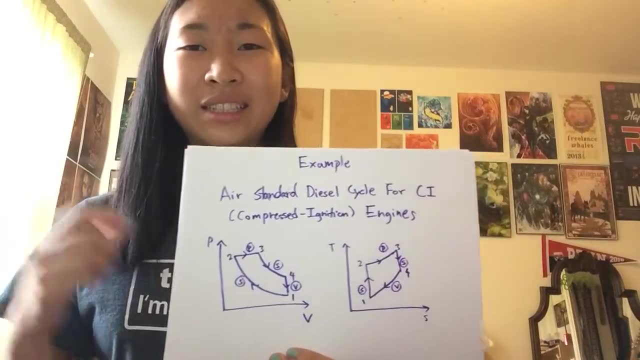 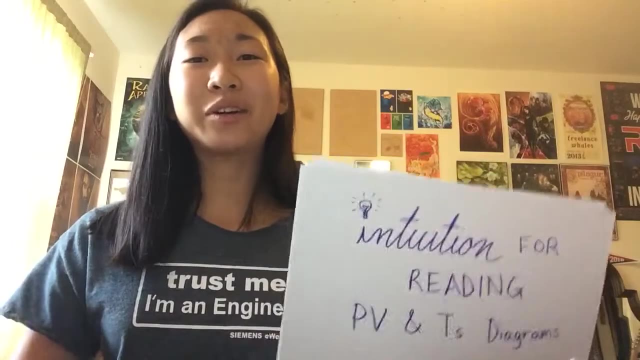 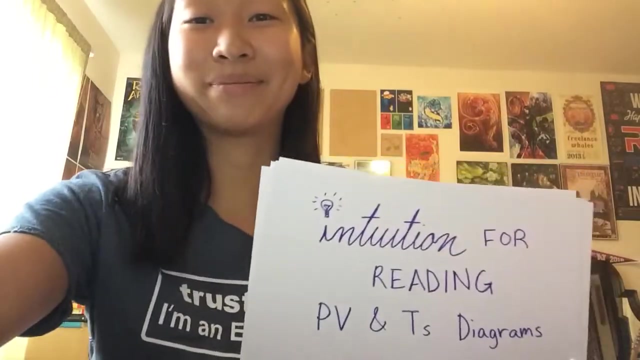 and properties of this cycle and the processes with mathematical expressions. but the basics are right here And that's how I would read PV and TS diagrams and explain them, without all of the equations or trying not to use all of the numbers. Okay, I hope that helped. 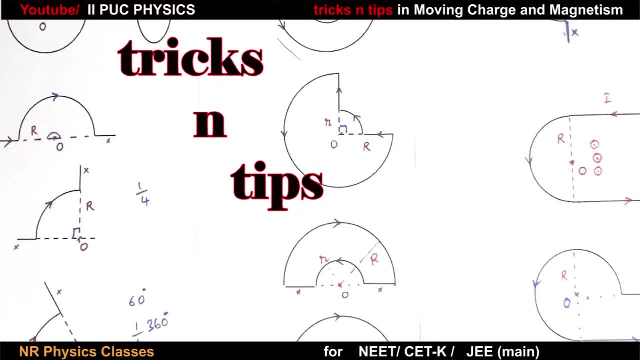 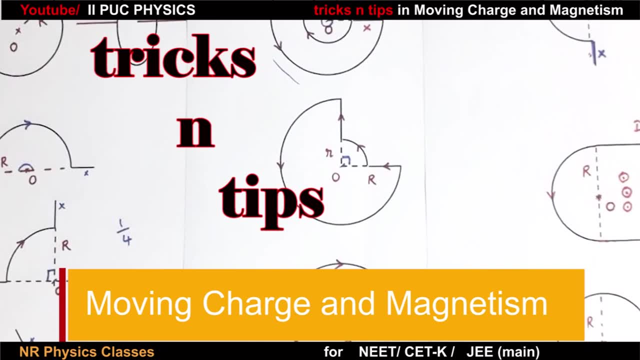 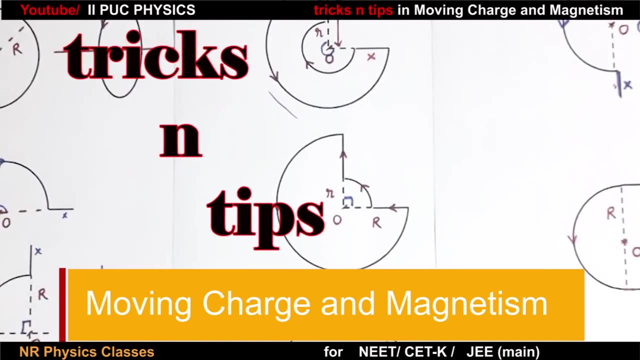 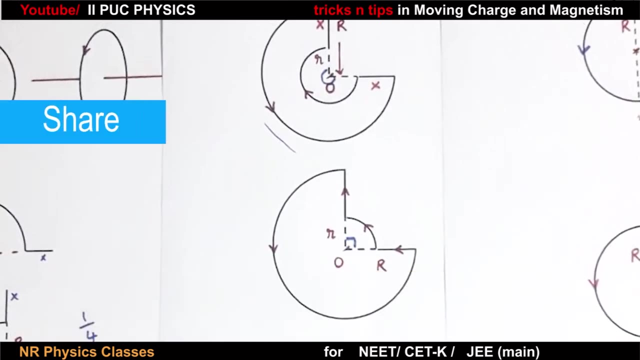 Hello students, in this video on moving charge and magnetism, let us learn how to find magnetic field due to conductors bent into different shapes. Such questions have appeared in all level entrance examinations: engineering, medical, BSE and MSE. MS. Kindly share like. 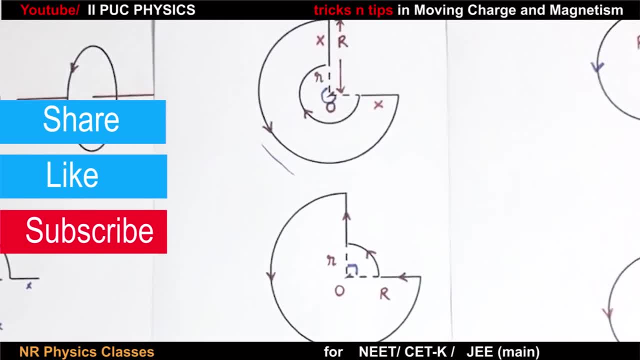 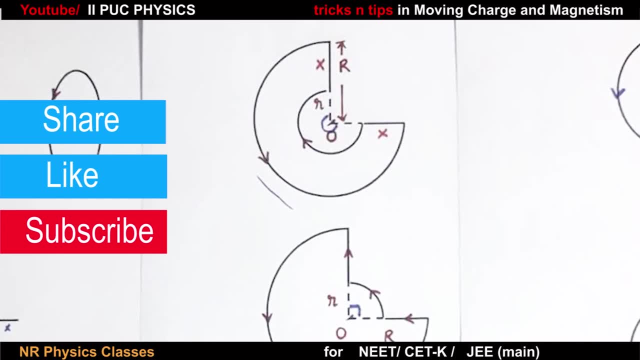 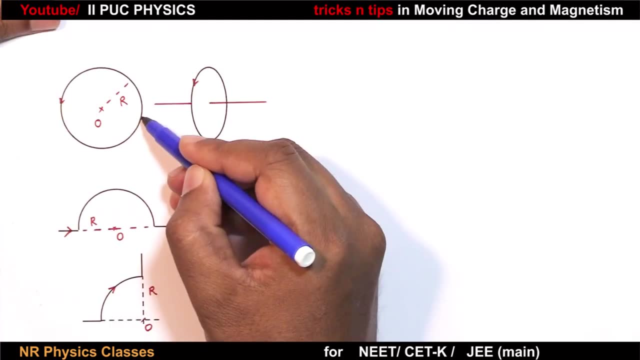 subscribe and press bell button for notification on future videos on time. Share it. share it in WhatsApp, Facebook, Instagram till it reaches students in rural areas who have no access to resources. Thank you, Circular coil radius R current through the coil is I. 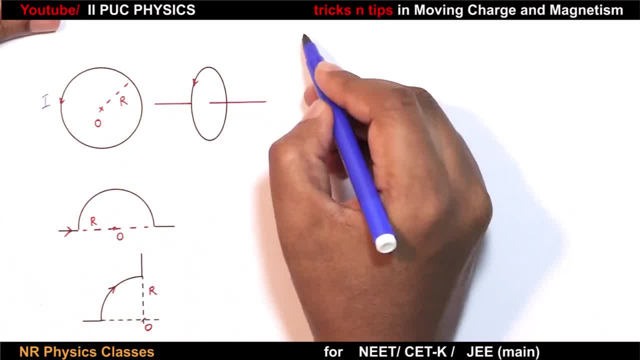 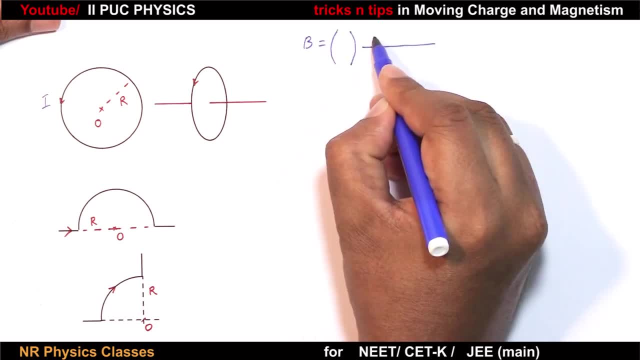 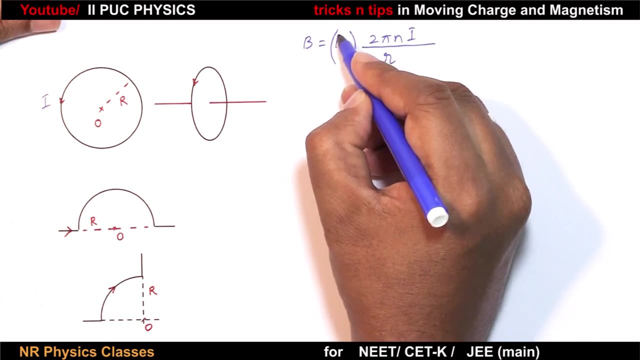 Magnetic field at the center of the circular coil. So magnetic field is given by constant 2 pi n I by R. This constant in magnetism is mu naught by 4 pi. If you simplify this further: 2 pi 1, 2 pi 2.. So this is mu naught n I by 2 R, Constant 2 pi 1, 2 pi 2.. If you simplify this further: 2 pi 1,, 2 pi 2.. So this is mu naught n I by 2 R Constant: 2 pi 1, 2 pi 2.. If you simplify this further: 2 pi 1, 2 pi 2.. So this is mu naught n I by 2 R Constant: 2 pi 1, 2 pi 2..